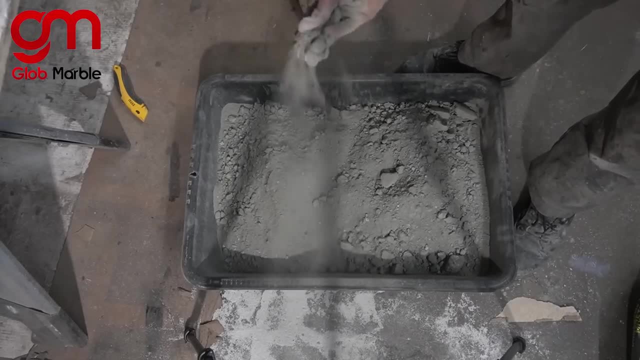 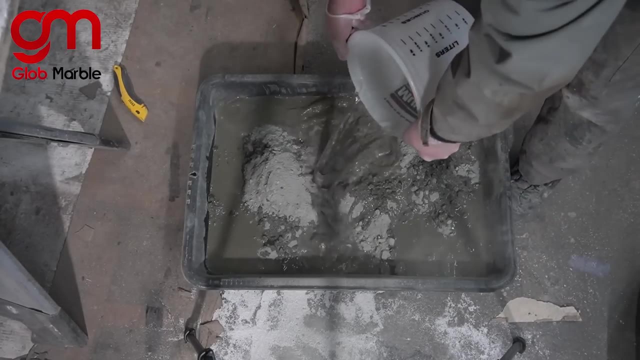 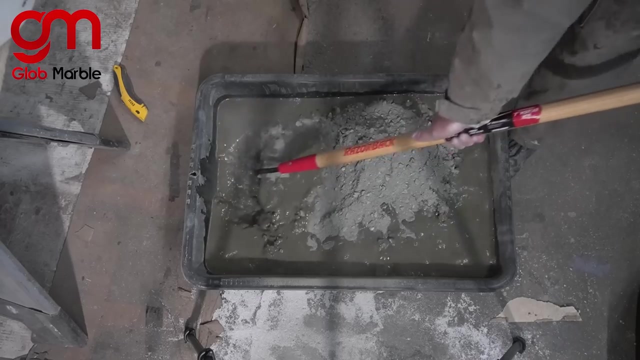 but if you can kind of crush it in your hands, it's not that big of a deal. Take my three and a half quarts, dump it out. Don't try to make a puddle, Make it sort of even. Take my hoe and start mixing it in until you can't find any dry clumps, dry spots. 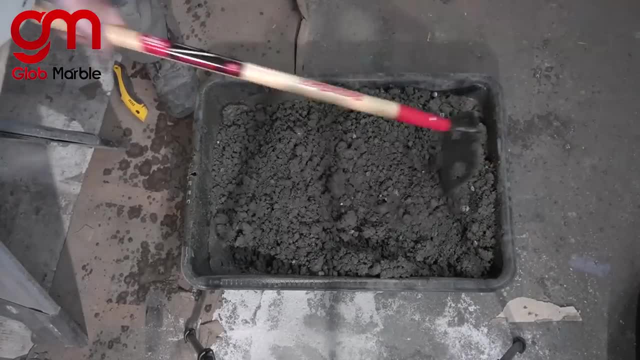 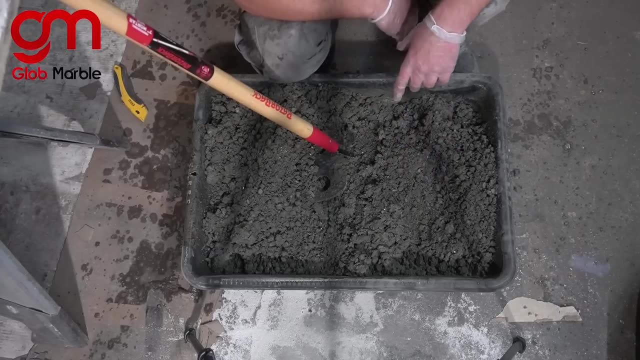 I don't like the consistency too much, so I'm going to add one more quart to see if that makes it better. But don't add too much water, because the more water you add, the weaker the concrete gets. I'm not that worried right now by adding another quart, because this is the high 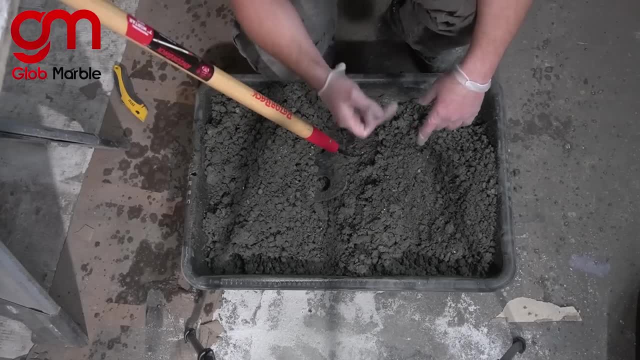 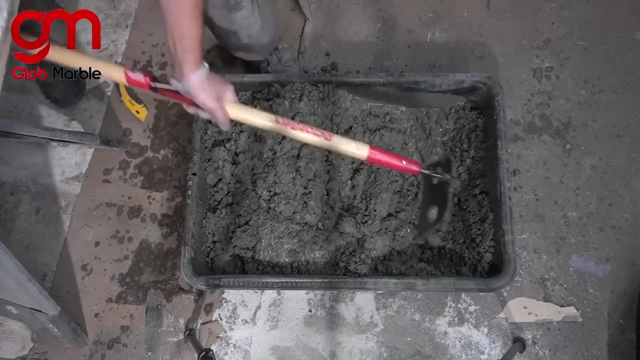 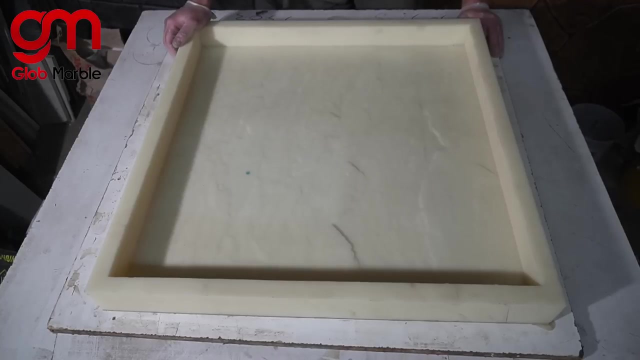 strength mix. Let's just see what happens. Globe Marble molds are made out of polyurethane, not silicone. The advantage is that polyurethane is way more durable. Our customers say that they've casted thousands of times without it breaking. You can't get that with silicone. The ironic thing is that it's also cheaper, So our products are. 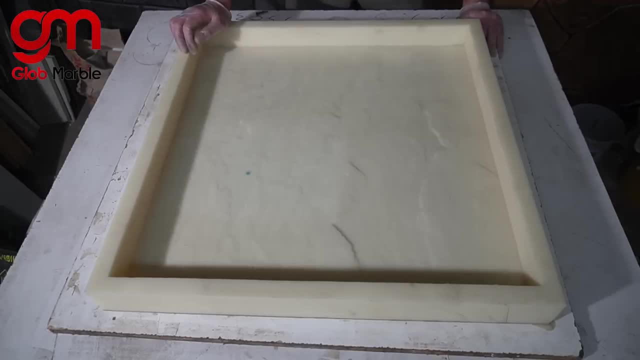 cheaper and more durable at the same time. That also means that you have to use a release agent. You can't just pour it straight in here, where the concrete won't release, won't get out of the form. Our release agent is G1. It's highly concentrated. You dilute it with water. 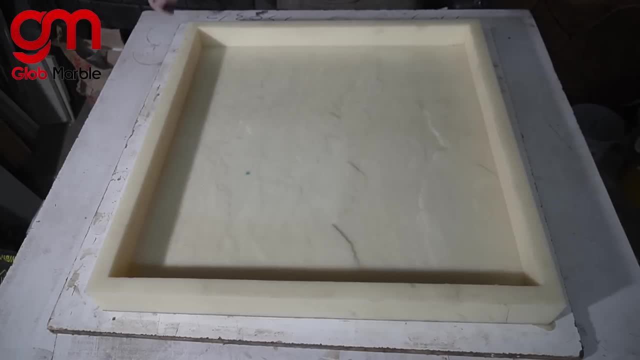 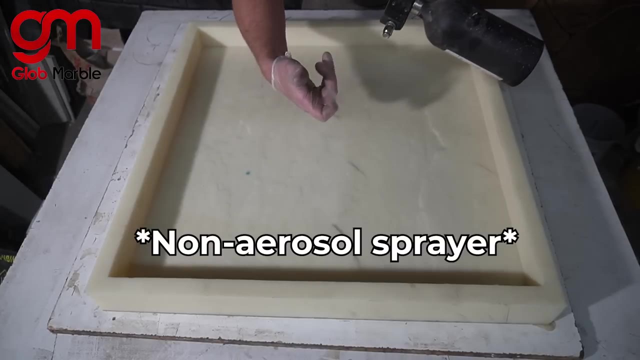 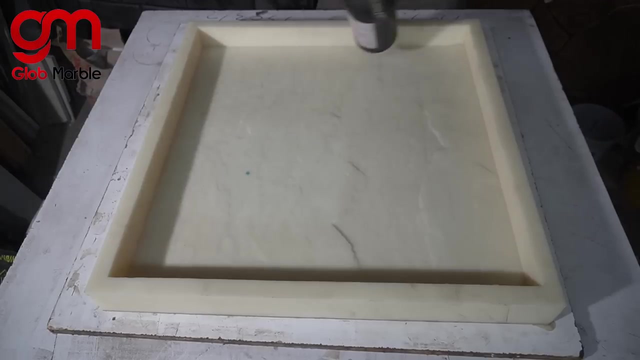 You can use it for a really long time for lots of casts, and you can use it in a regular sprayer also, But I like this one because it sprays way finer of a mist than you could get with the squirt bottle, and that makes you use a lot less of it. Again, you don't need a lot. I'm spraying a light mist. 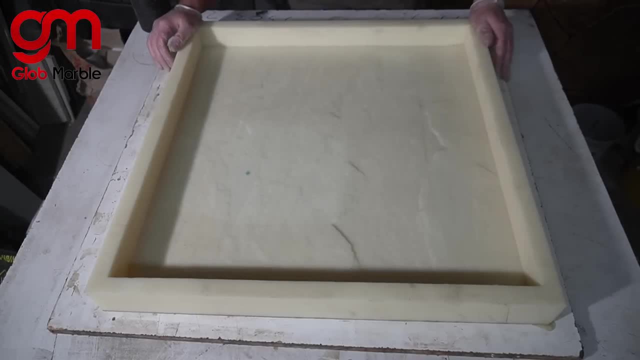 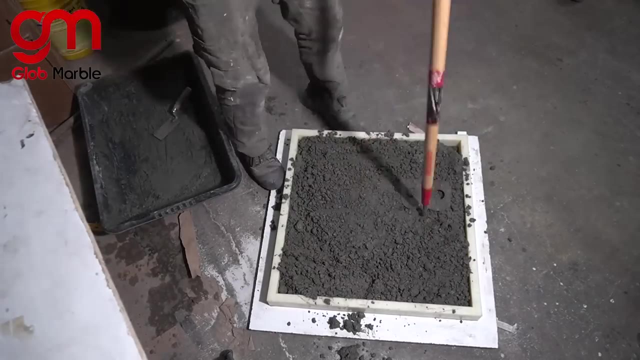 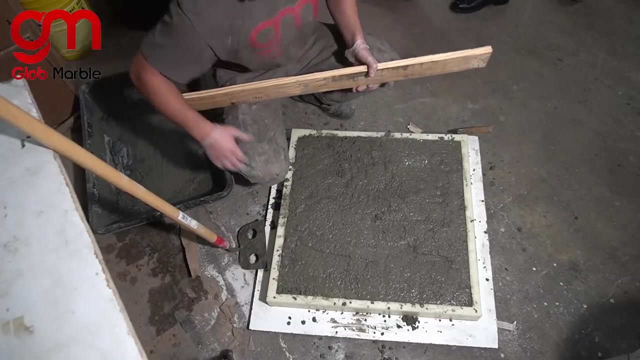 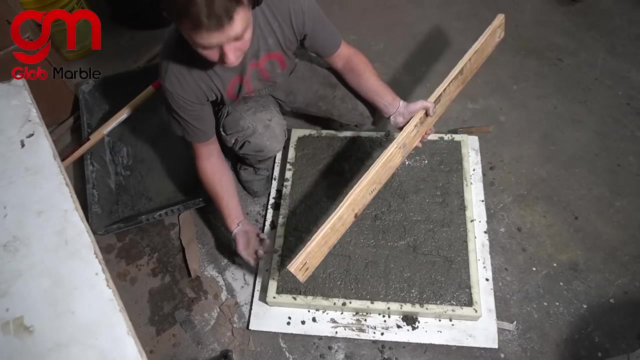 And I'm done. I'm going to move this down to the floor so it's easier to pour the concrete into it. So we got some low points over here, so we're just going to take a regular plank of wood and then screed over the top of it to remove everything that's above the form walls and then put the. 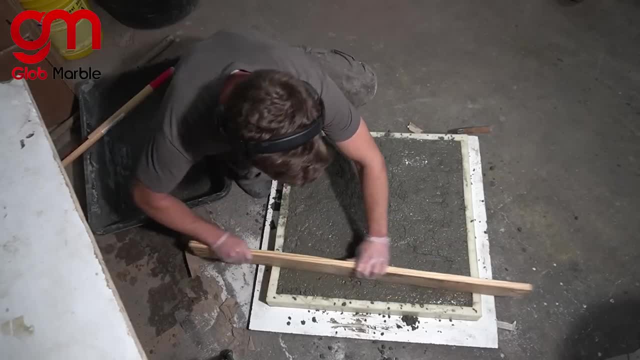 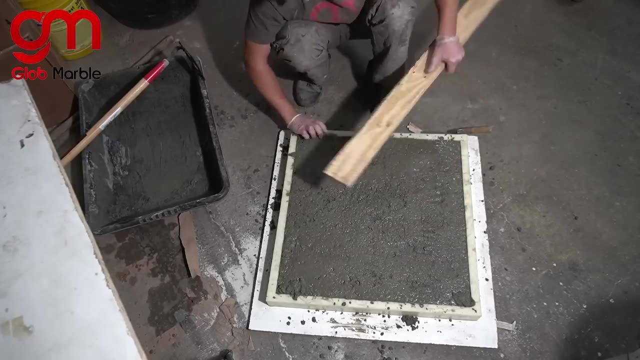 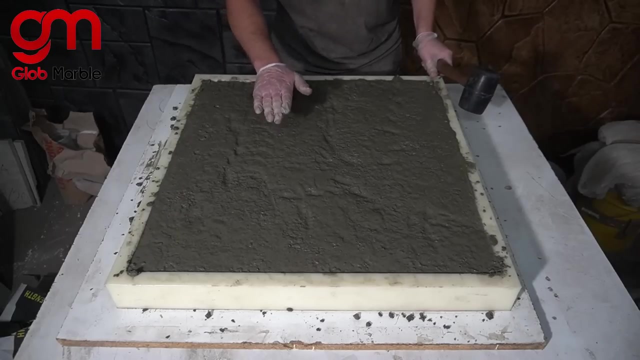 excess into those pits over here And now it's time to get rid of the bubbles on the surface, where the actual stone texture, where you're going to be walking, what you're going to see, is going to be, Because the concrete was a little bit dry, there definitely are going to be bug holes. 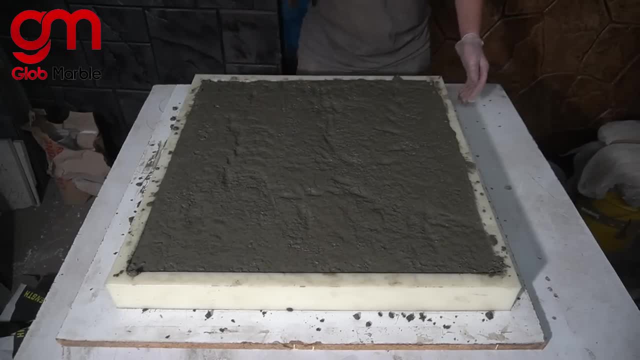 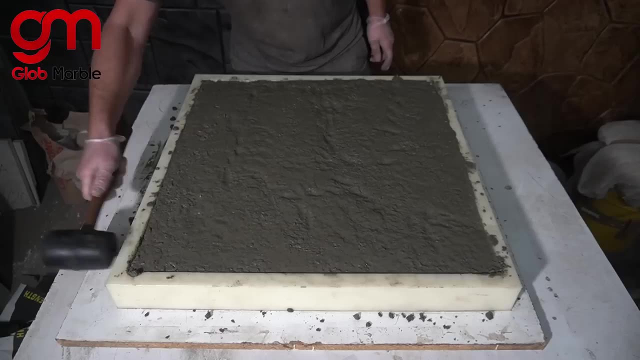 but this is how to fix it. I'm just going to take a rubber mallet, put it on top of a table and bang underneath the table and on the sides, Do the sides first, because they tend to separate like this If you leave it like that. 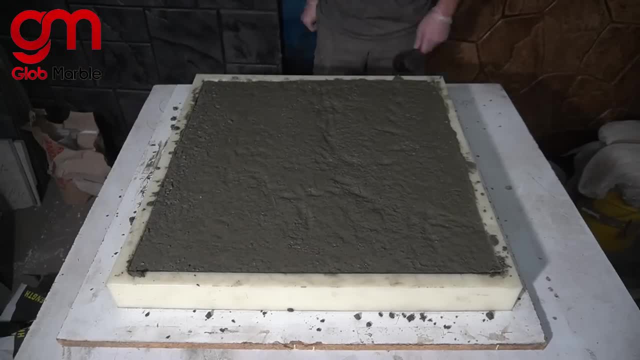 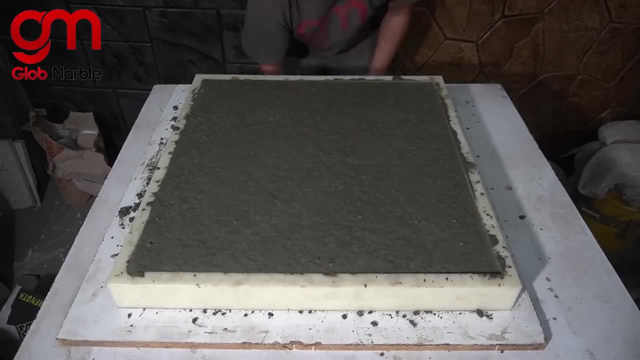 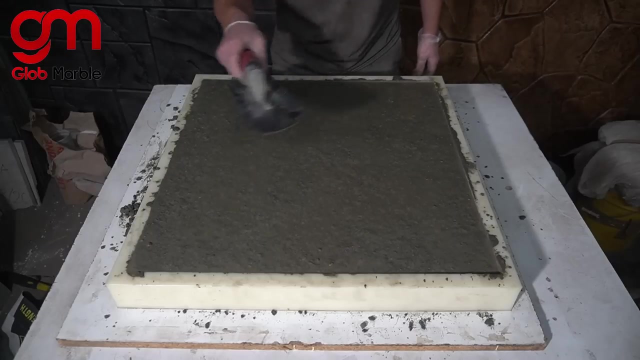 it's not going to be a good look once it's all finished And now you don't need to do this, but I like to. It looks a lot nicer even though you're not going to be seeing it. But I'm going to take a pool trowel. 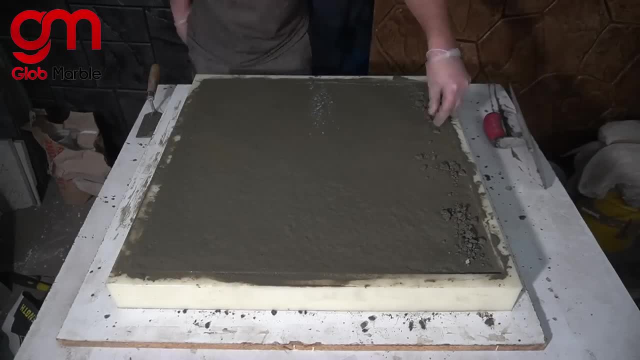 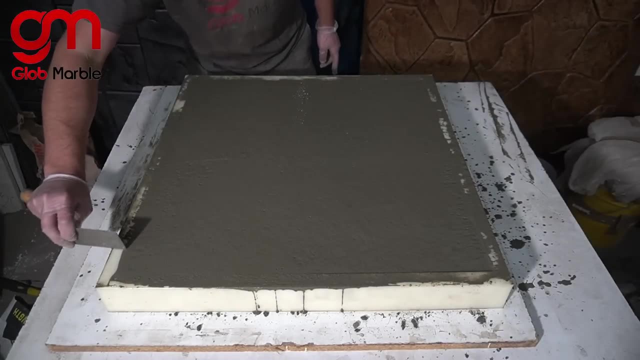 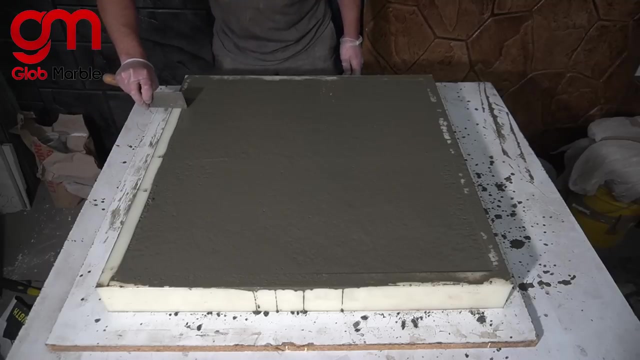 to smooth everything out And once the concrete is still fresh. it's a lot easier to clean off the mold right now than it will be once it dries up. So I'm going to take advantage of that. clean everything off. It's going to make your mold last for a lot longer. 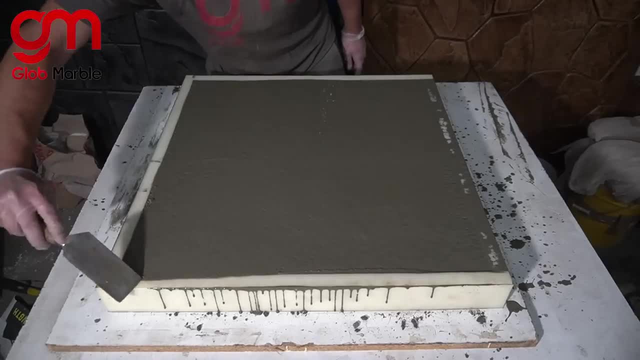 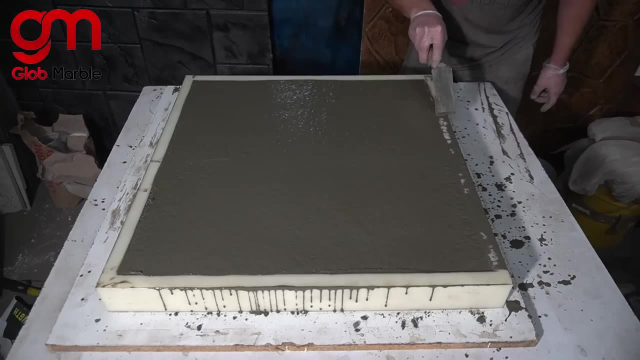 And then we're going to cover it with a piece of plastic. You do that so that the concrete doesn't lose too much moisture. You don't want it to dry too quickly while it's curing, and that's going to make the concrete a lot stronger. 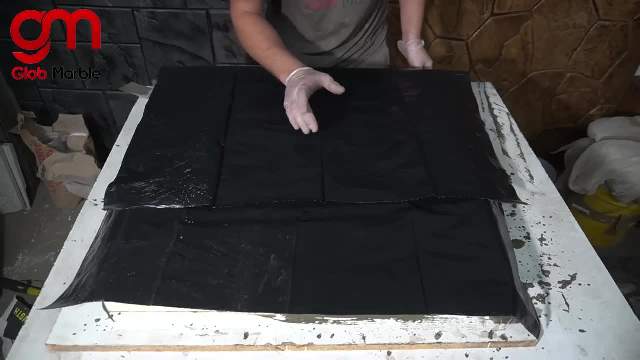 Now, even though it's winter, I can't afford to demold this tomorrow because I'm inside and the place isn't going to be that cold overnight. If you're working outside, you definitely want to wait two days before demolding. If it's really really cold, it involves heat. the same way. 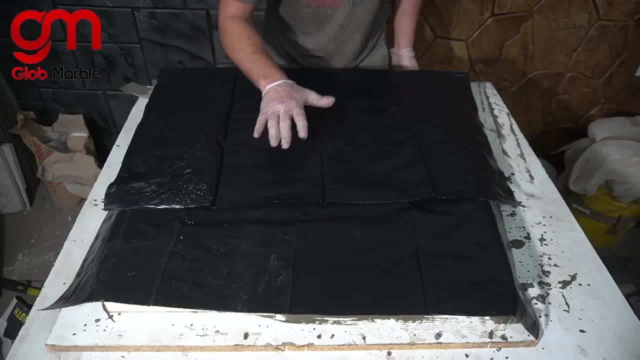 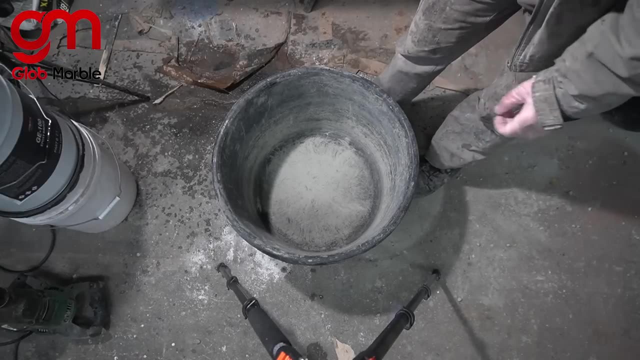 but vice versa. If it's really hot outside, your concrete is going to set up a lot quicker. Even though that first method was really cheap, it's still really time consuming and labor intensive, And so for the rest of the other molds, I'm going to be doing this method. 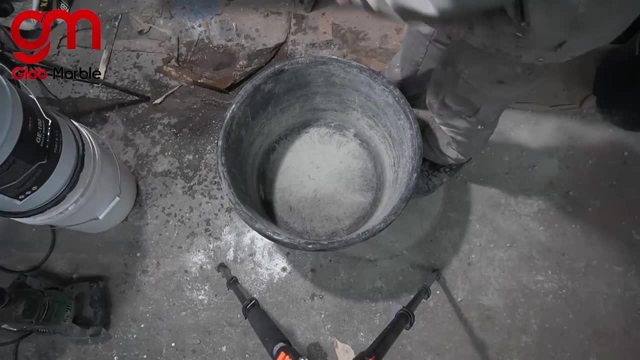 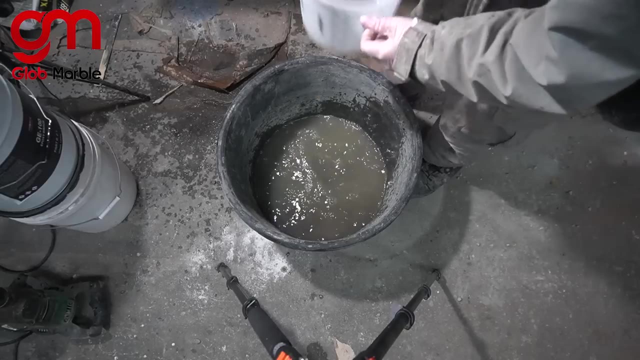 First we get a bucket instead of a trough, And we already know from experience that it's best to put four and a half quarts and put the water in first, all of it down to the bottom of the bucket, And now we're going to pour half of the concrete out. 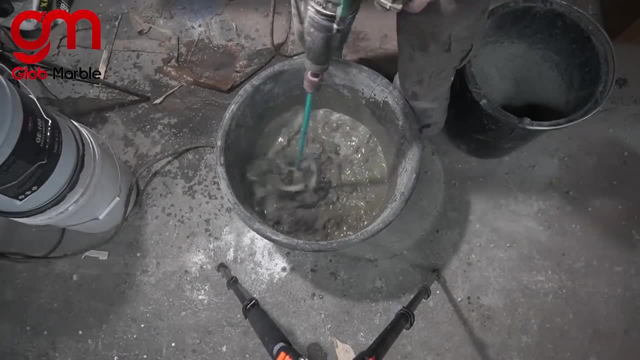 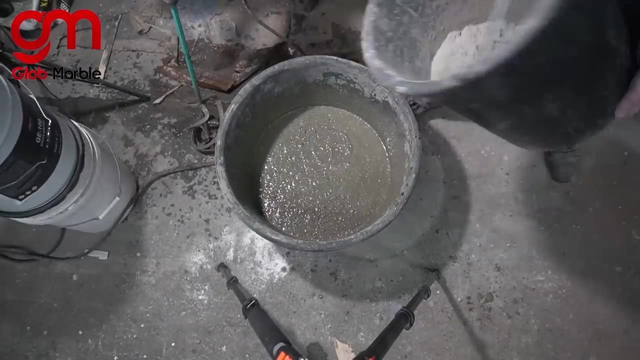 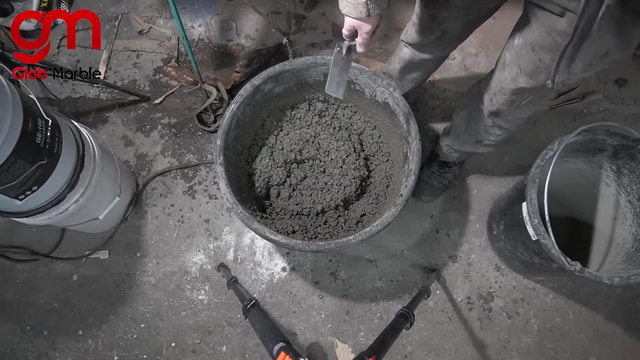 and use an electric hand mixer to mix everything in And then pour the rest in. The reason we did it in multiple pours is because it's just way easier to be able to get all the water dispersed evenly across everything, So some spots don't stay dry. 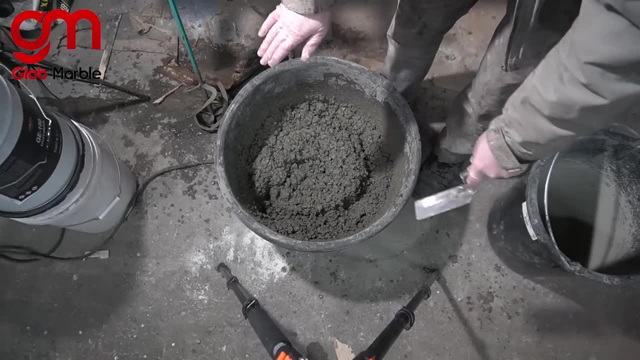 and some spots don't, So we're going to pour half of the concrete out and use an electric hand mixer to mix everything in. We're going to pour half of the concrete out and use an electric hand mixer to mix everything in, So some spots don't stay way too wet and slushy. We've got everything as even as possible. 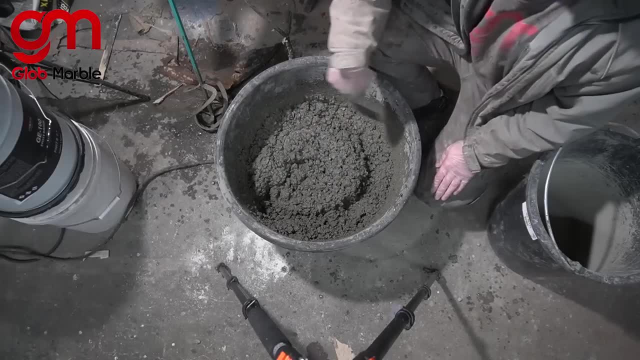 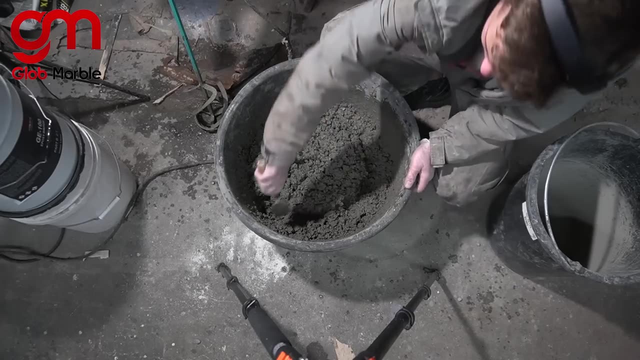 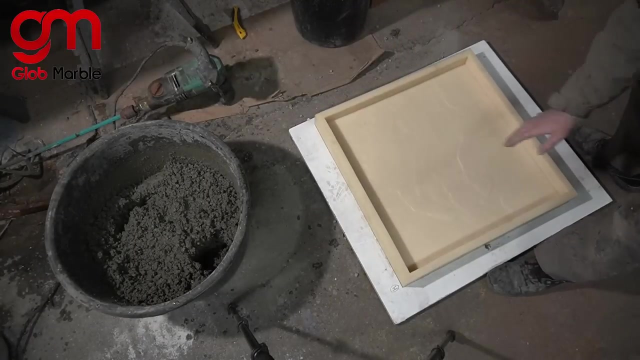 Now we're going to take our hand, trowel and scrape the sides of the bucket to make sure there's no dry material left over on the sides. Then we're going to mix it one more time and then cast. And now you've seen how I use a melamine board to be able to transport everything around. 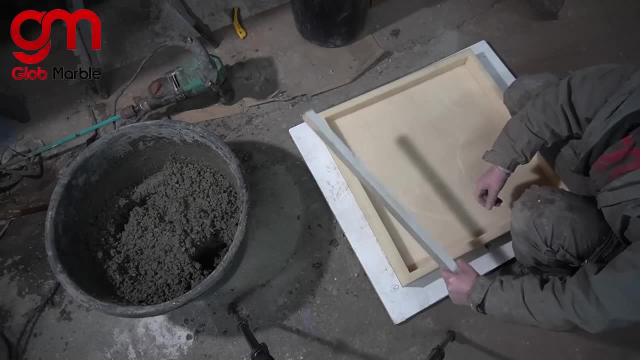 Before you do that I forgot to tell you. Before you do that I forgot to tell you. Before you do that I forgot to tell you- Place a stick underneath one side of it, just so that you have a good spot to put your fingers under and pick it up. 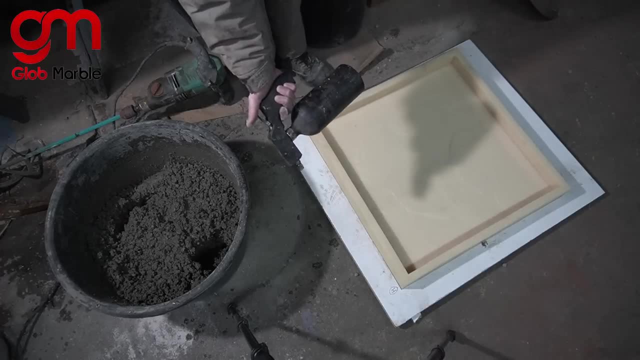 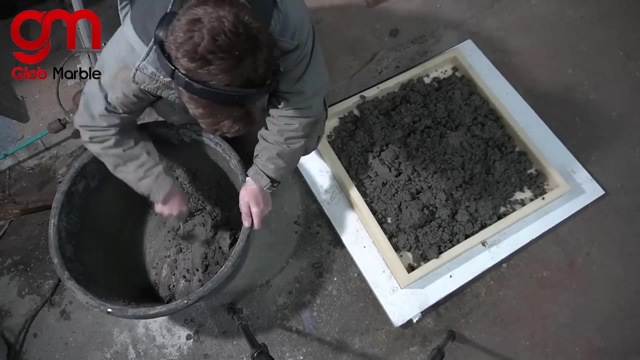 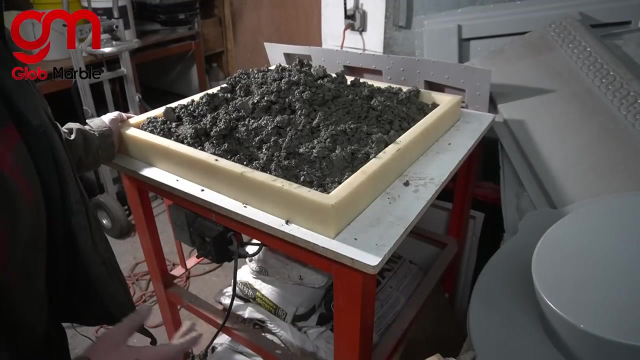 instead of trying to lift it and pry it from the floor Again, we spray on our release agent And now, instead of sitting there and tapping it with a hammer- which doesn't always work and is pretty time consuming, labor intensive- I'm going to put it on a vibration table and then 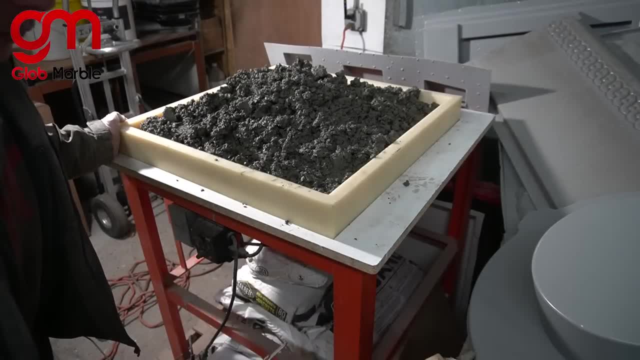 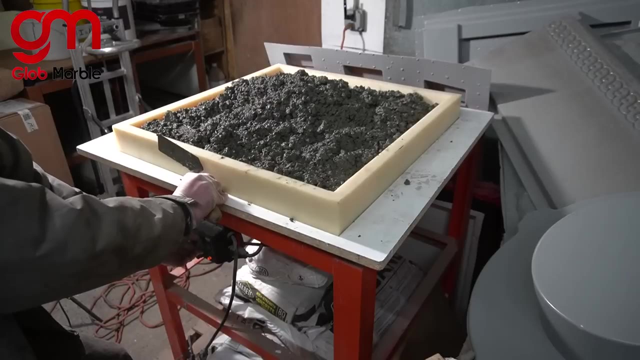 vibrate it like that, These could be a little bit more expensive. If you want to make a makeshift vibration table with just the motor, you can. I'm going to link a video in one of the corners of your screens right now. So 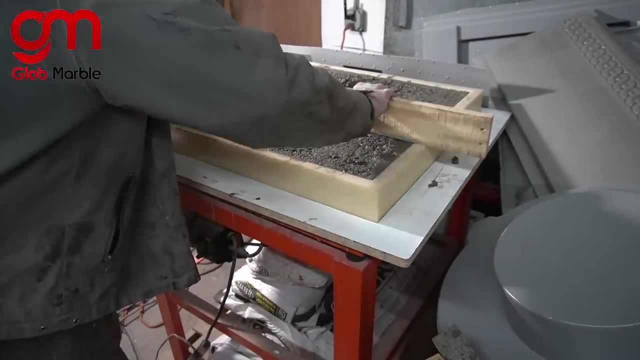 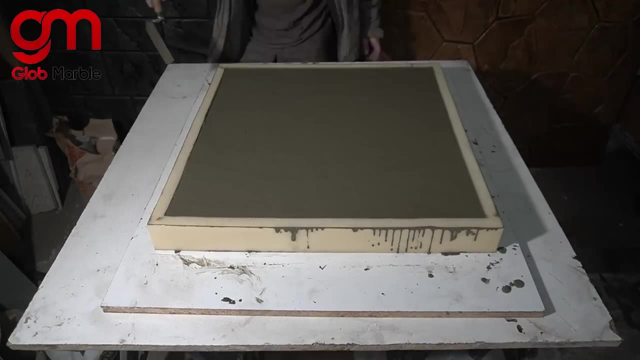 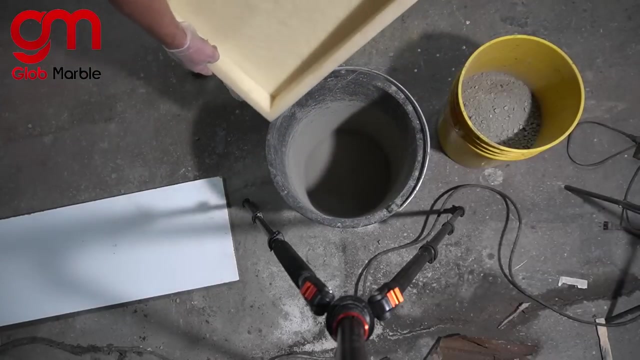 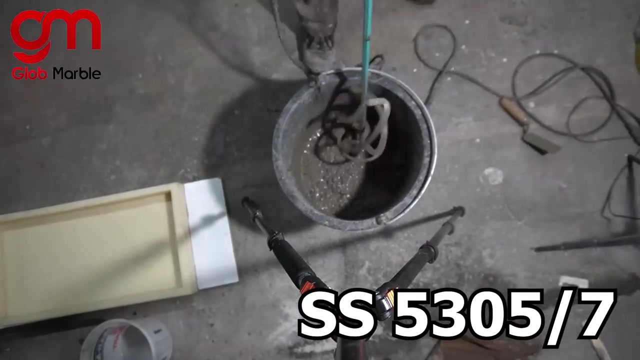 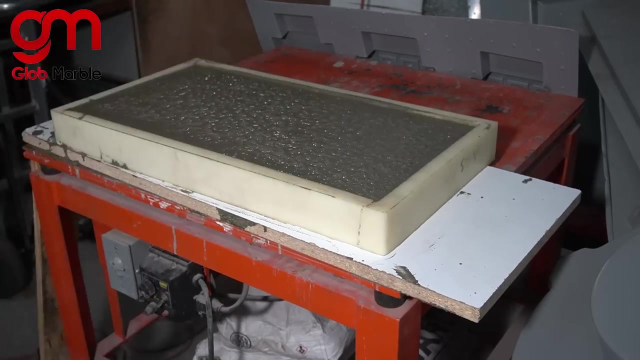 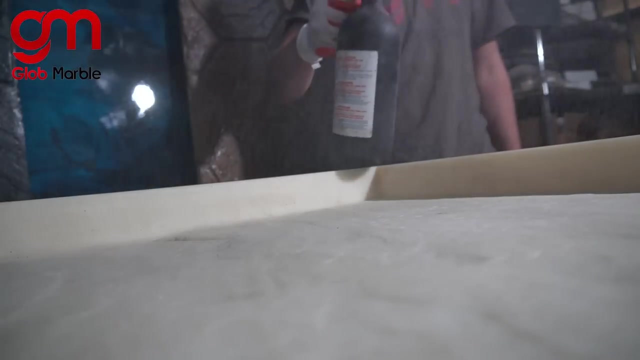 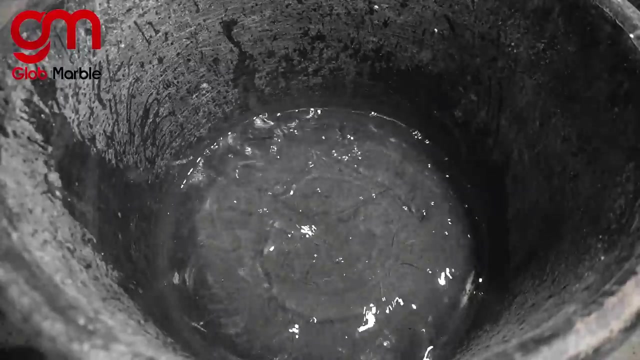 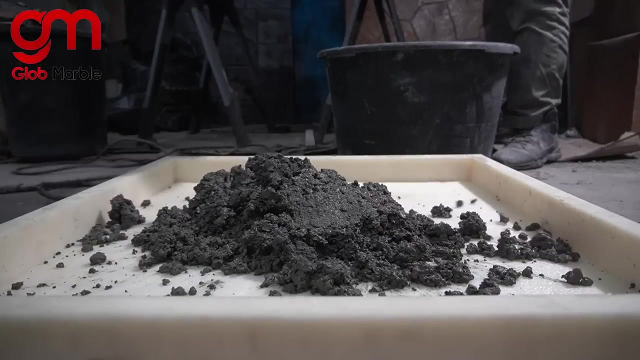 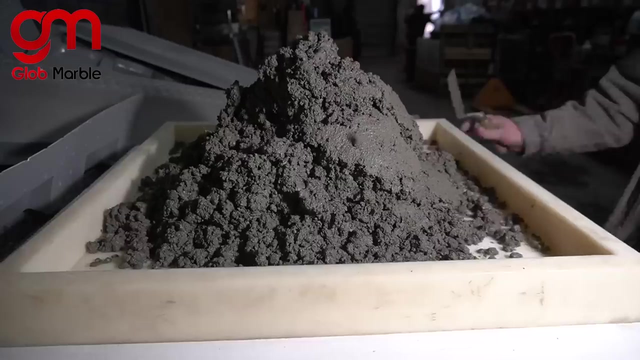 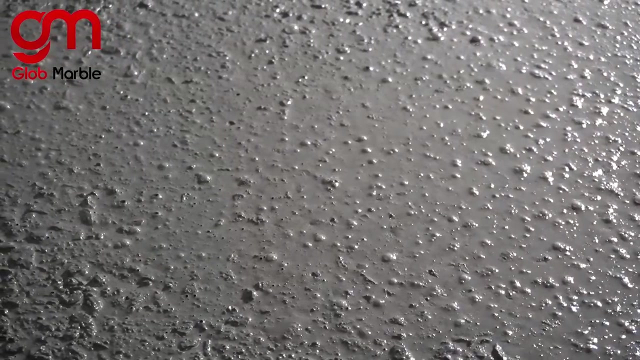 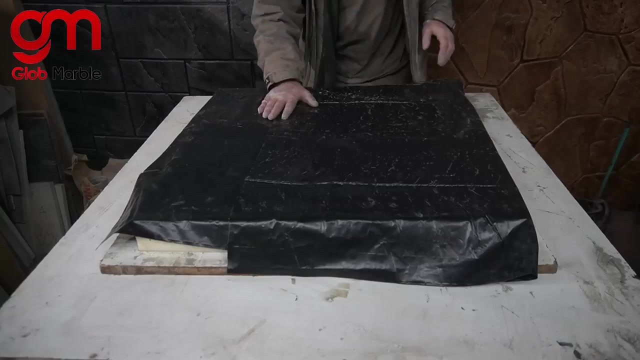 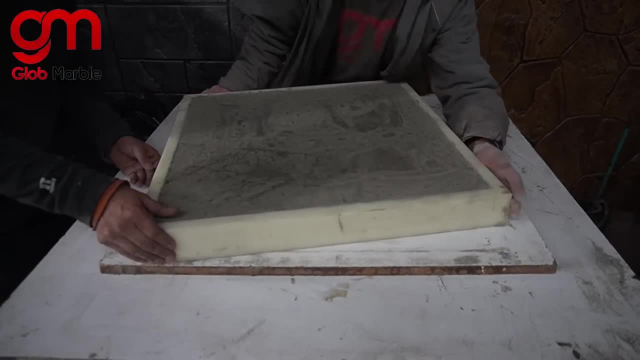 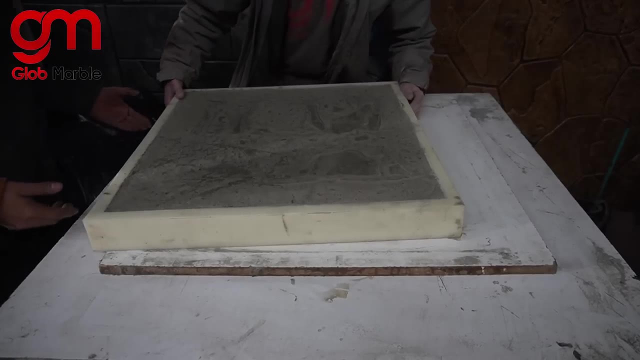 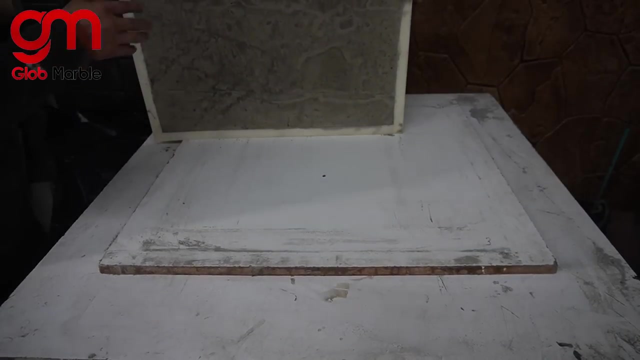 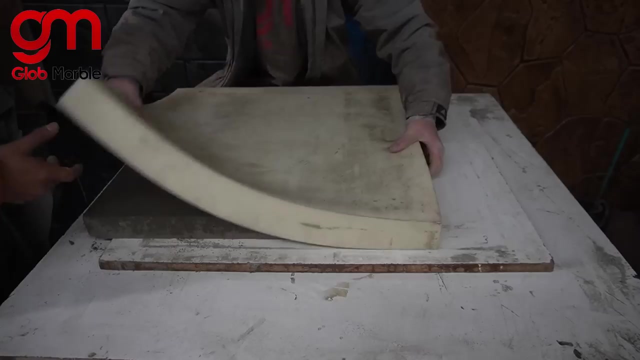 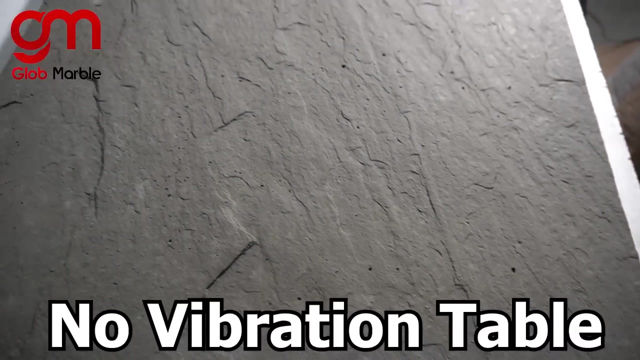 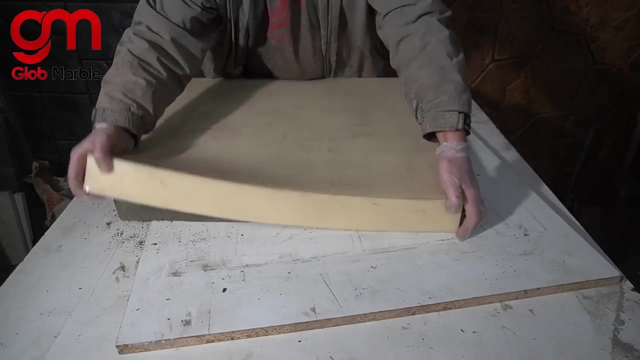 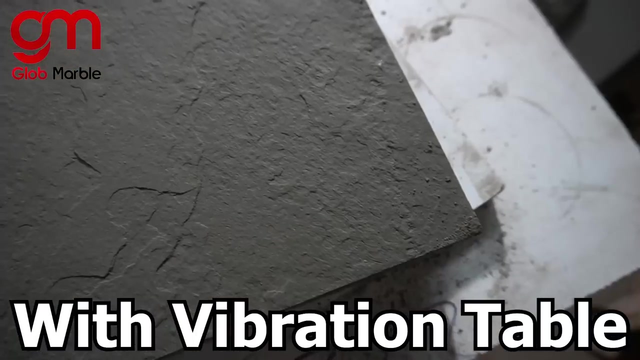 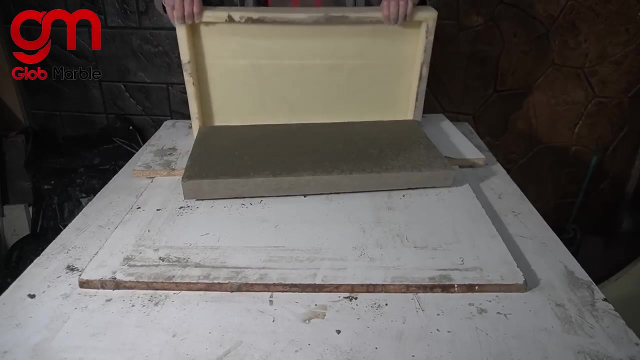 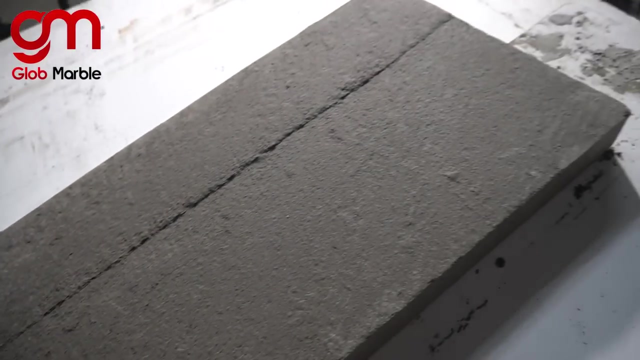 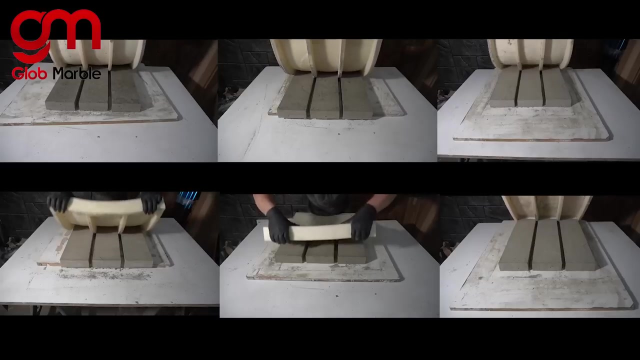 I'm going to move this over over the edge of the plywood- I mean the melamine- so that when I demold it and drop it it's not going to catch my fingers underneath there. There we go. And then I also casted SS5303-4 and 5303-5 for my border stones. 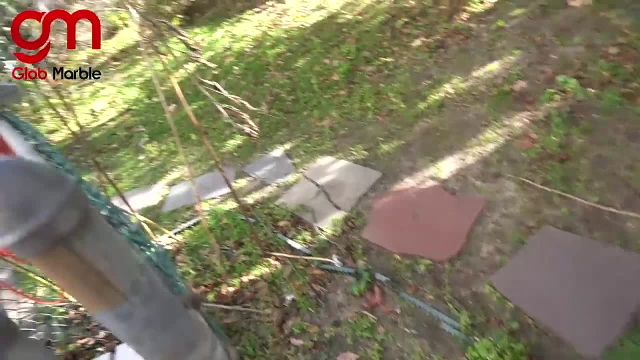 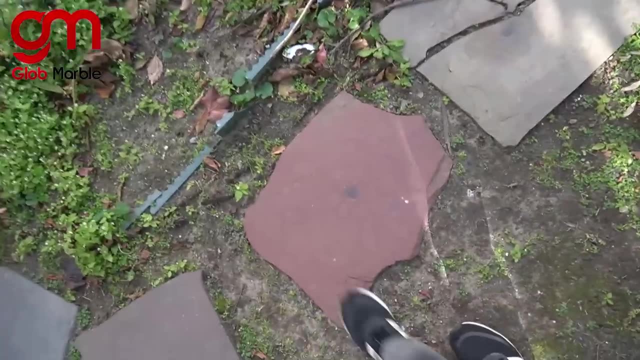 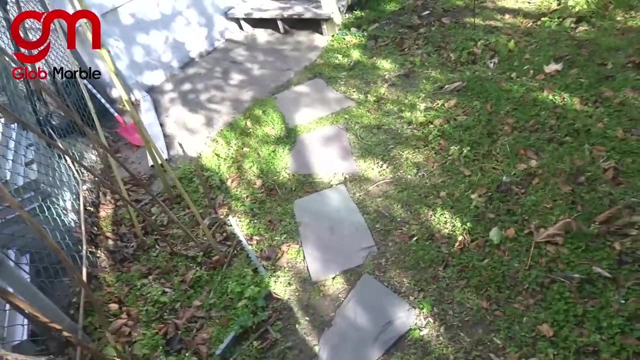 So now it's time for the installation. I'm going to remove these stones that were here Beforehand and most of the time you're going to have almost like it is right here where it's not really elevated too much, And basically what guys do is they go ahead and they dig a hole and put the pavers inside. 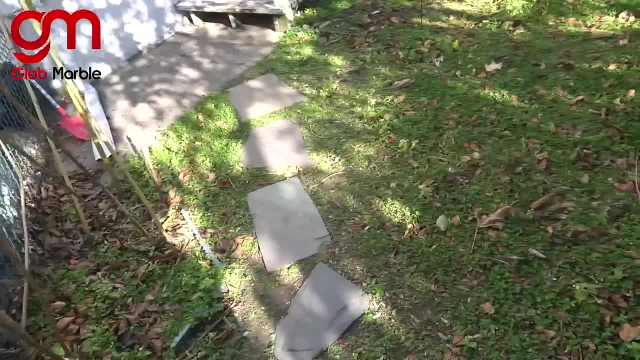 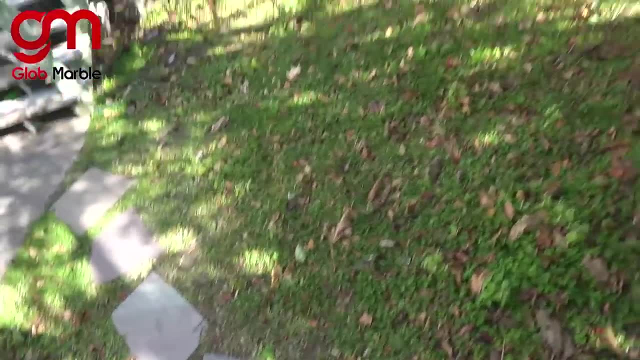 of the hole that they dug. But I'm not going to do that because around here there's a bunch of dirt and grass and every single time it rains, this gets all muddy. So I'm just going to have it elevated to make sure that that doesn't happen. 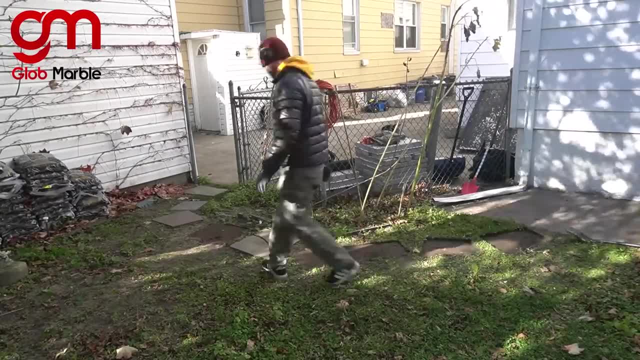 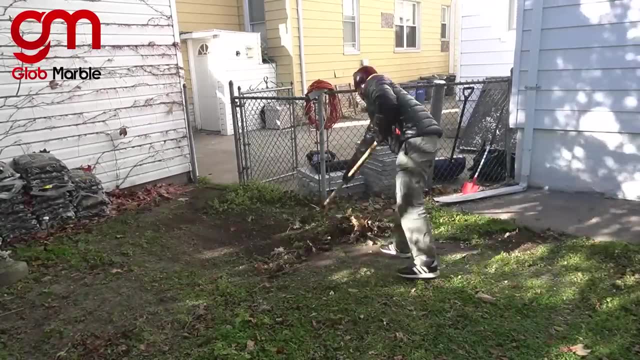 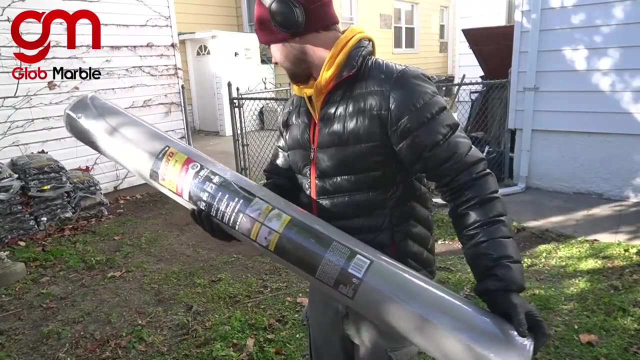 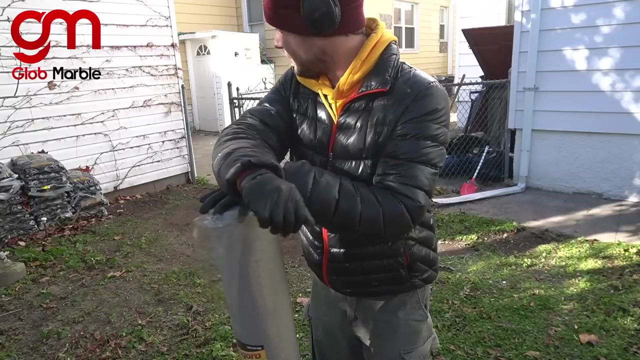 Now we're going to have to set something up called a weed control fabric. Basically, what that does is it stops weeds from growing in between the little stones we're going to be putting in between the paving stones. It's going to keep this looking nice for a lot longer. 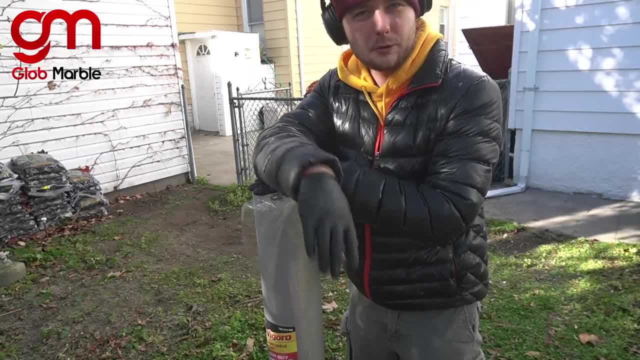 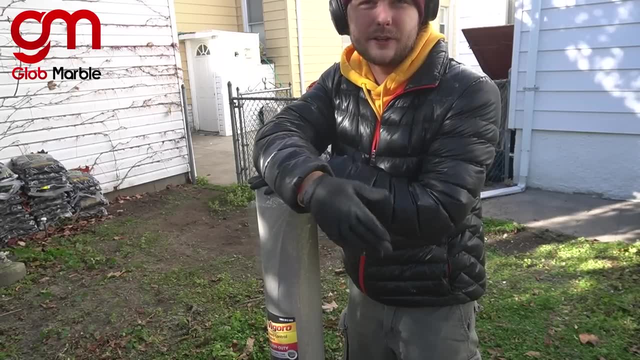 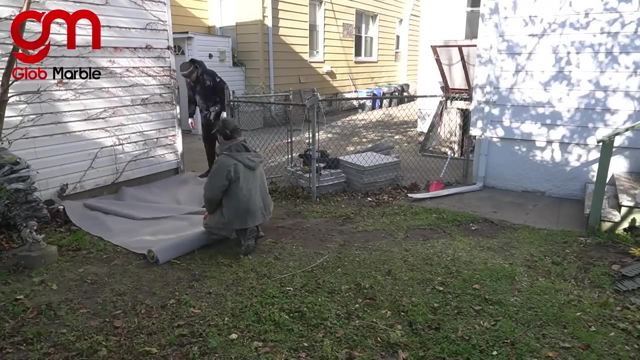 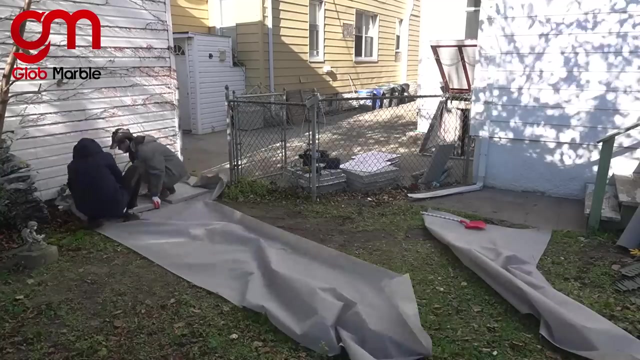 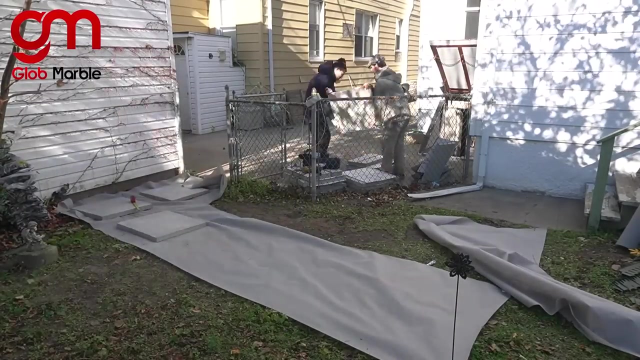 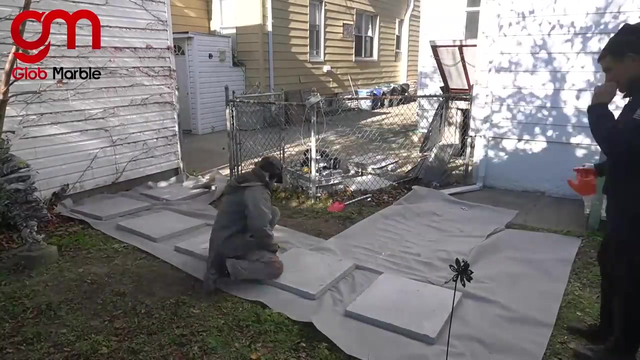 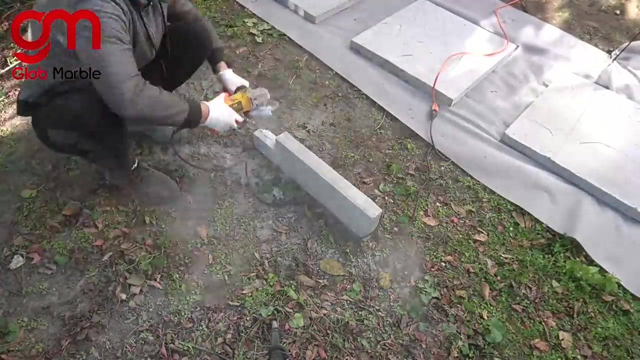 I'm just going to lay it down onto the floor and, after I've already placed down all of the stones that I need to place, I'm just going to cut around the edges everything that's extra, And that's going to be how we're going to do it. 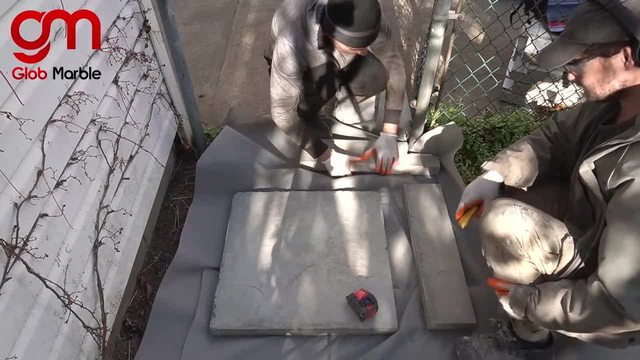 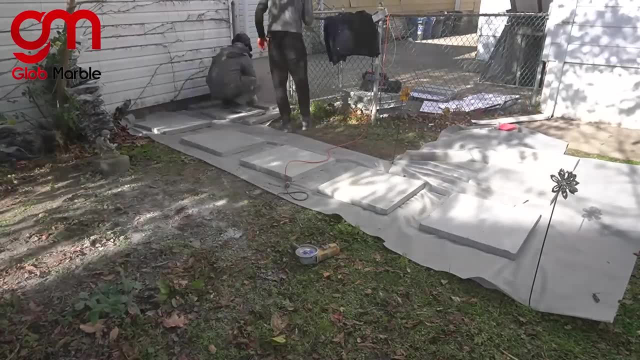 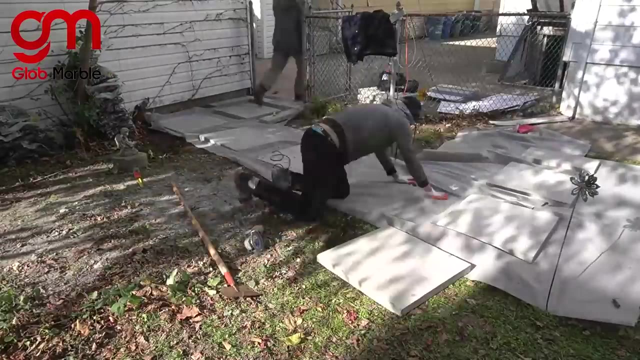 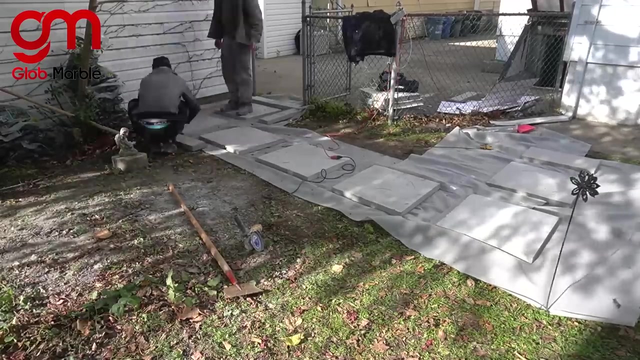 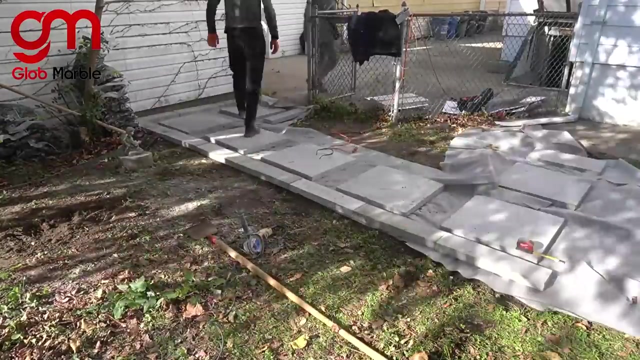 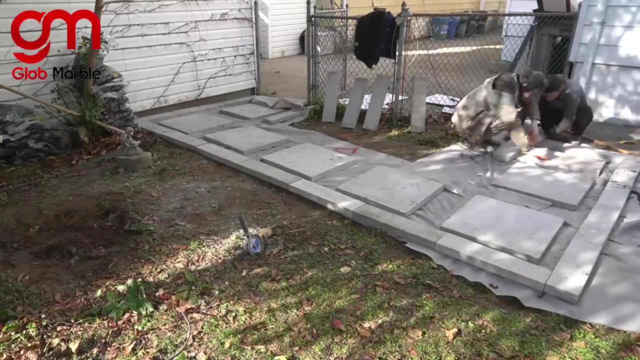 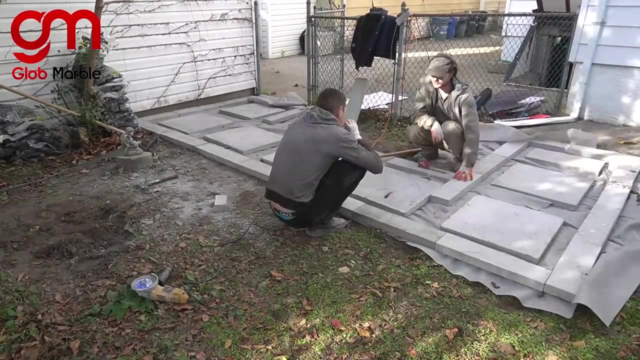 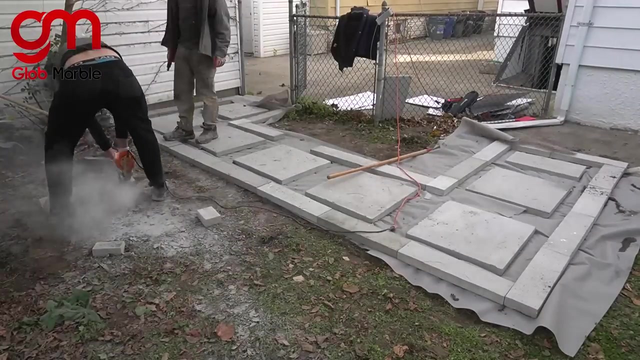 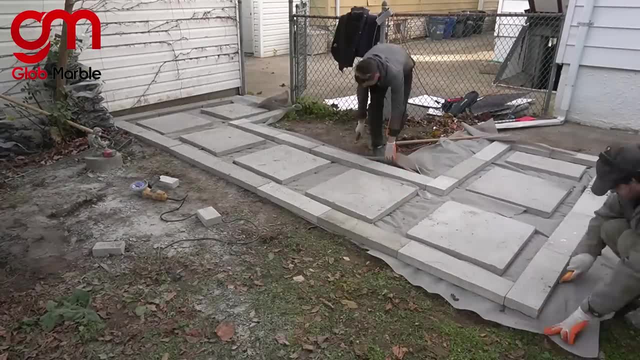 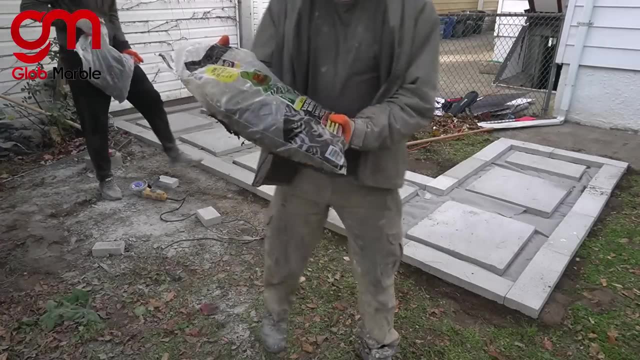 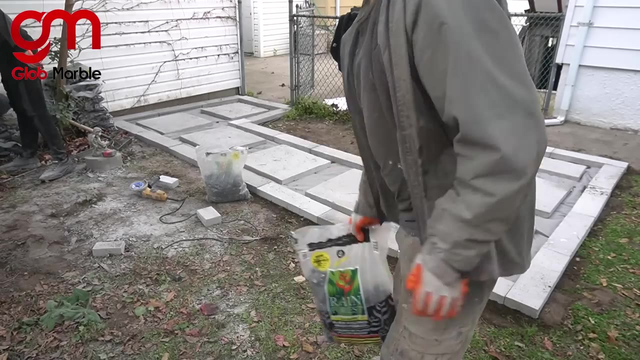 Then it's time to pour the river stones. Now we're going to go ahead and grab our black polished river pebbles. You can see it's not even half a square foot per bag. That's terrible, but they're going to look really nice.